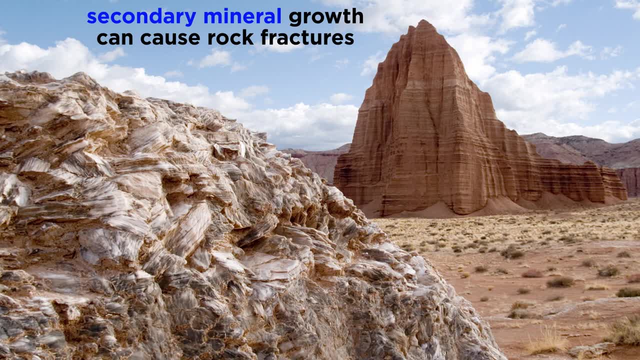 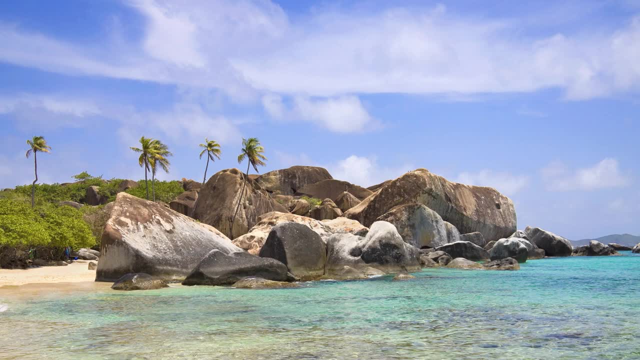 fractures such as gypsum or other salts, has a similar effect to the freezing of water we just mentioned. Tropical environments do not experience much physical weathering. however, they have intense chemical weathering due to abundant precipitation and high temperatures. Physical weathering also has a biological effect, which is the effect of the freezing of water. The 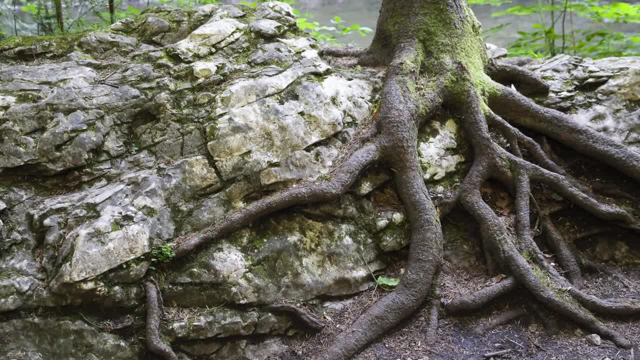 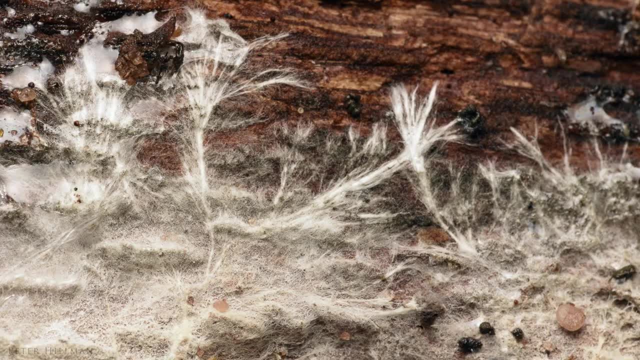 temperature in the arid regions of the world is also a biological component. For example, the growth of tree roots into small rock openings can widen and open them into larger fractures. The branching root-like hyphae of fungi have a similar effect. The burrowing of animals like moles can bring 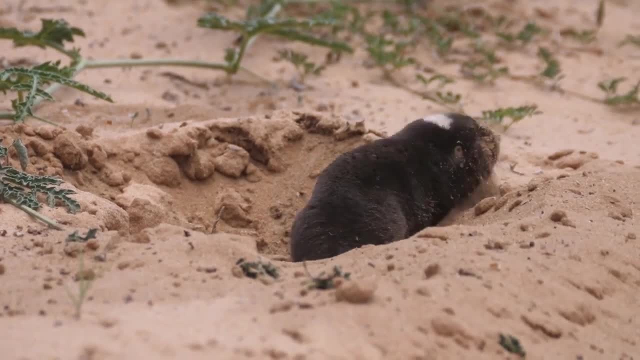 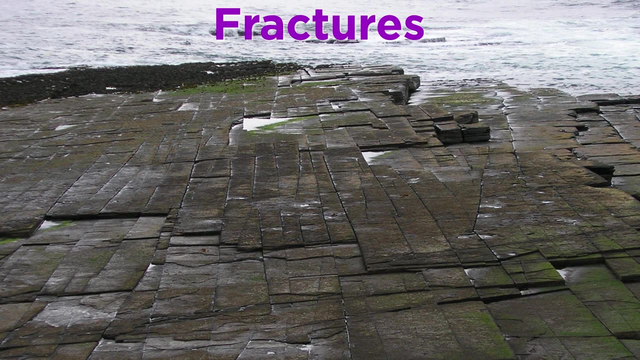 fragments of rock to the surface, where they are chemically weathered more rapidly. Though not considered weathering, the formation of regular sets of joints or extensional fractures in bedrock greatly accelerate the weathering process. All rocks can be weathered by the temperature of the 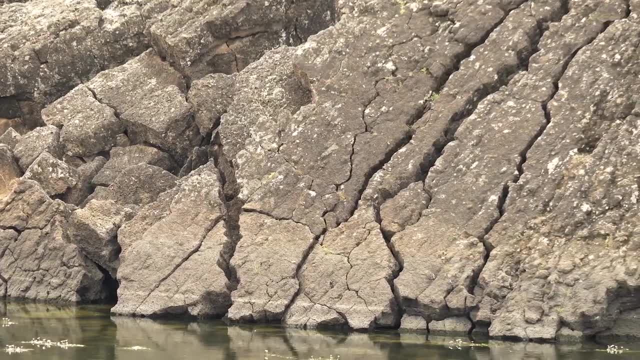 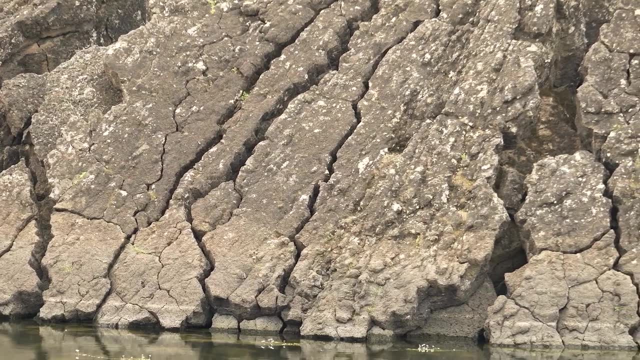 rocks, and they can contain fractures which form in a lined, perpendicular fashion to its least compressive stress. It is common for a geologic formation to form regularly spaced sets of joints as it is being uplifted to the surface and the stress field changes from a state of horizontal. 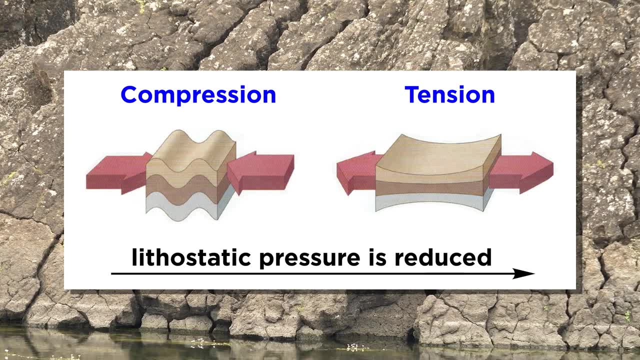 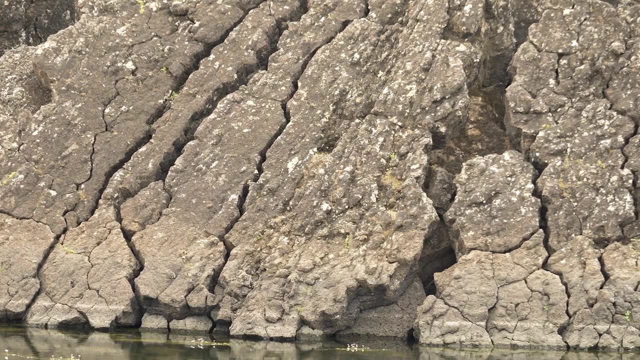 compression to horizontal tension as the lithostatic pressure or pressure from surrounding rocks is reduced. These joints tend to be perpendicular to the surface and occur in sets of two at around 90 degrees, and the pressure from the rocks is reduced to about 90 degrees per second. 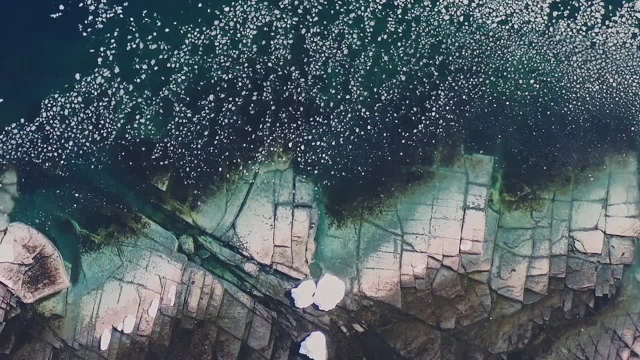 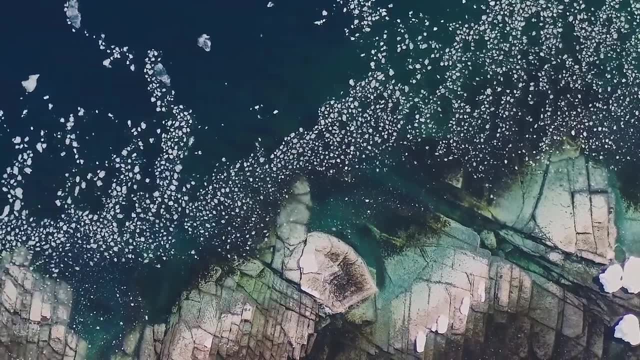 Though they can be much more complex. Next time you are driving along the highway, notice how nearby rocks are broken along planar surfaces, forming a step-like pattern. That is not the work of humans, but of mother nature. At any rate, joints provide starting areas for the other. 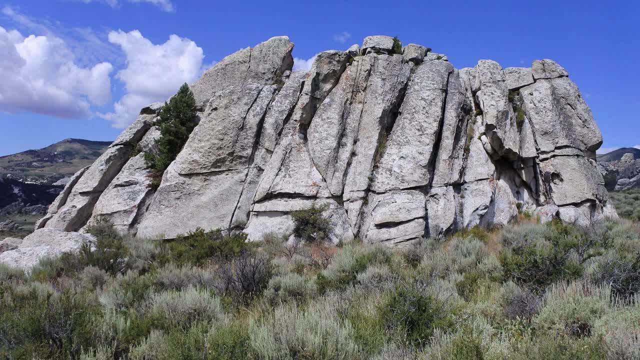 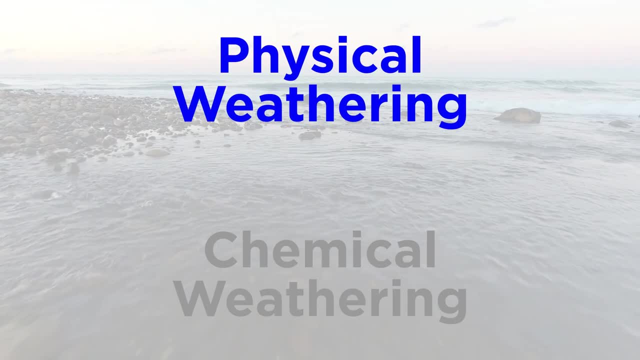 mechanisms of physical weathering to operate and since they're often filled with groundwater, they make great areas for thirsty tree roots to enter in search of water. With physical weathering covered, let's move forward and take a look at the next section. 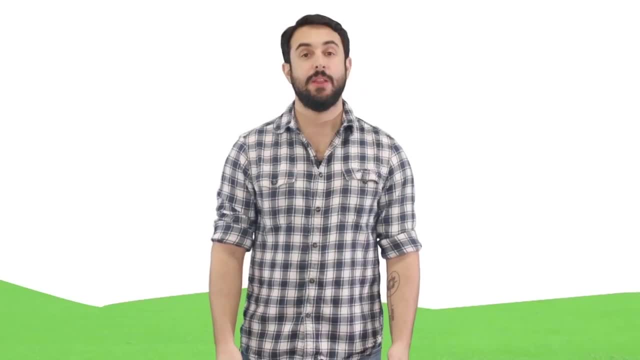 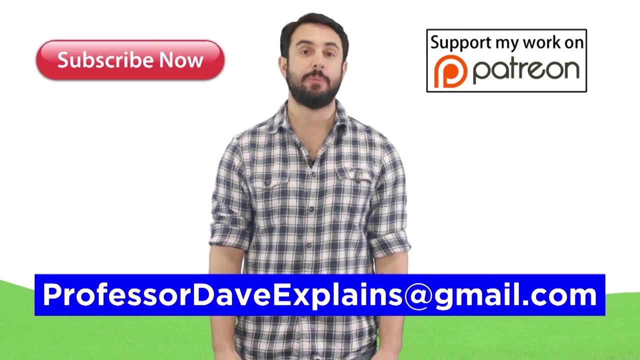 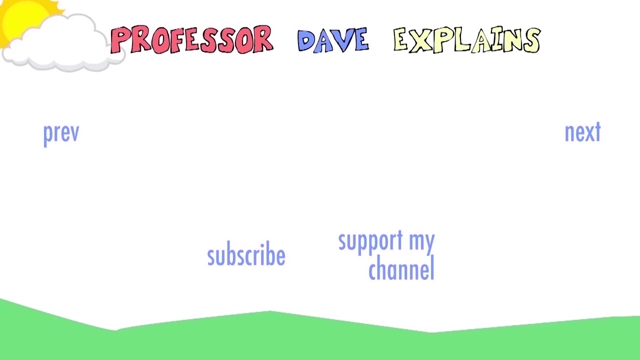 Thanks for watching. Subscribe to my channel for more tutorials. support me on Patreon so I can keep making content and, as always, feel free to email me professordaveexplains at gmail dot com. I'll see you next time.